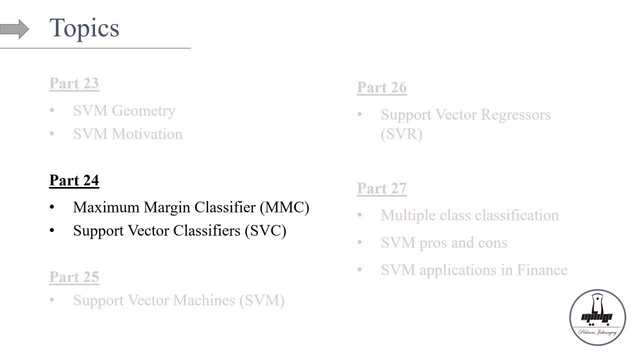 And we're going to do it in the classification setup First, and later on we're going to expand the idea for regression. So let's start with the definition of hard margin- MMC- maximum margin classifier- and soft margin- SVC. 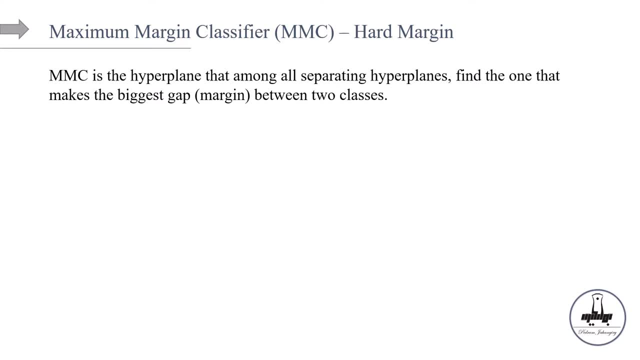 Okay, starting with the hard margin, MMC, maximum margin classifier. So MMC is a hyperplane that among all the separating hyperplanes out there we'll find the one that makes the biggest gap, the largest margin between two classes. So let's look at a classification problem. We have X1, feature 1, feature 2, and classes are two classes, basically green and red. So let's review some terminology here. This line is going to be our maximum margin, hyperplane or maximum margin classifier. The dashed lines are going to be our margins. So the observations on the margins are support vectors. So here we have two support vectors. 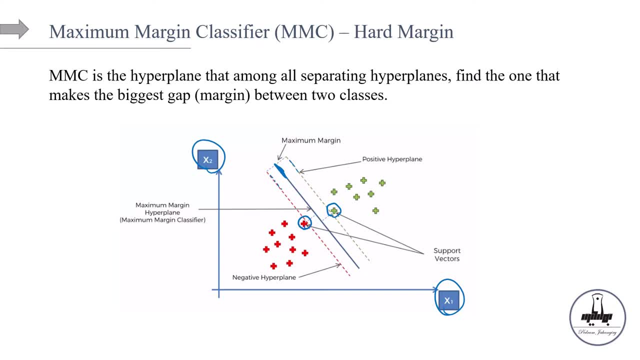 And the finally, distance between these support vectors are going to be our margin, So we are trying to maximize that margin. So MMC, maximum margin classifier, is basically this hyperplane that maximize the gap between two classes. So why are we trying to maximize the gap in the train set? Because if you find a maximum gap of the observations of the classes in the train set, we hope that the model is going to do a decent job in the test set as well. 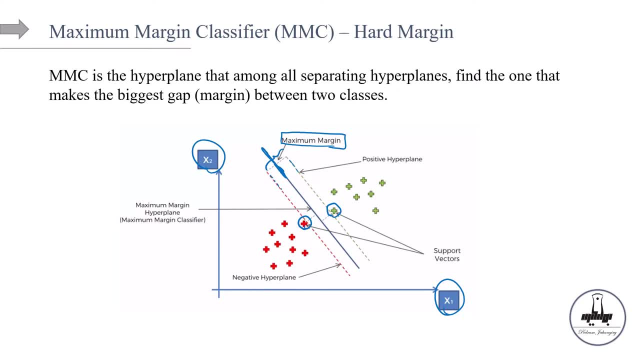 So that's why we're looking for the maximum gap. Okay, just remember that adding, you know, adding more training data away from the support vectors will not affect the boundary right. So if I add a bunch of red observations here, away from the, let's say, the hyperplane, or if I add a bunch of green observations here, it's not going to make any difference in terms of what is the functional form, what is the equation for the for the maximum margin classifier. 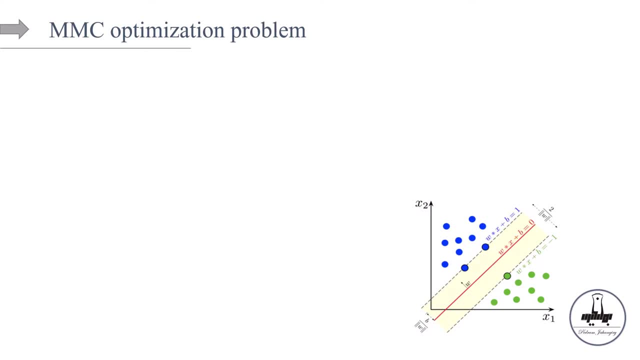 Okay, So let's do that. Okay, Now let's see how does MMC do the job. So what is the optimization problem? The core idea of a hard margin is to maximize the margin, the gap under the constrain that the classifier, the hyperplane, does not make any mistake, does not allow for any kind of misclassification within the margin right. 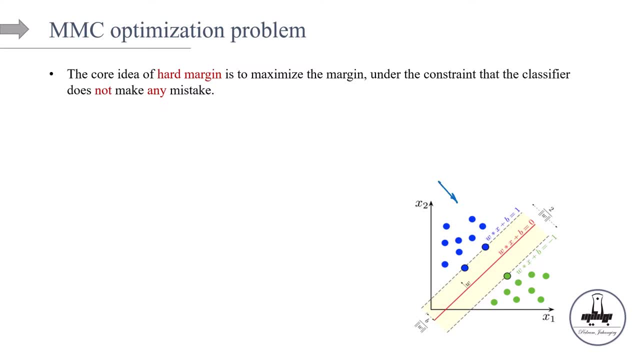 So let's look at this example. So it seems that if the red line is a is a hyperplane, the it's, it's, it's a, our MMC maximum margin classifier. it doesn't allow for any kind of misclassification, right. 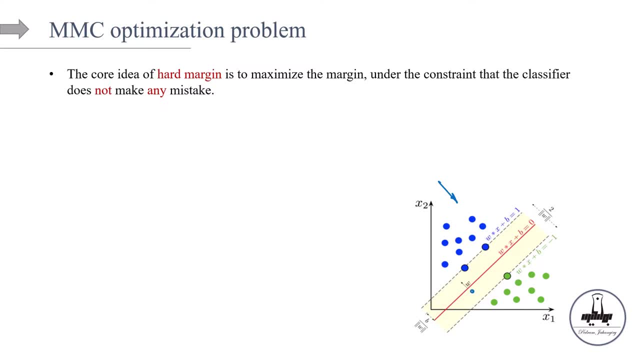 So let's say, if I had another blue observation here, because the blue observation is on the wrong side of the hyperplane, it's going to be misclassified, right. So, even though it's blue, but if I use this red hyperplane, the model is going to predict green, which we know that it's. 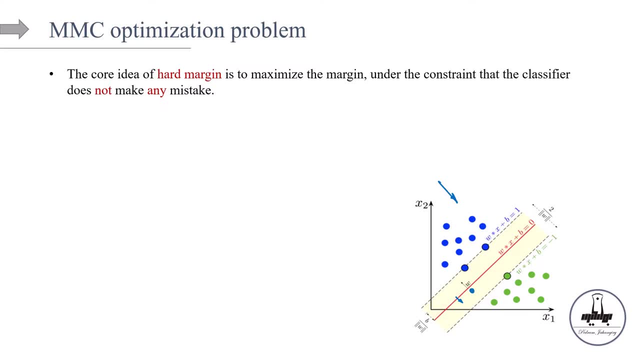 wrong. it's misclassified. So if that's the case and if you're using MMC, the new hyperplane is going to rotate in a way that the model does not allow for any kind of misclassification. So maybe the entire thing is going to rotate like this. So this is going to be the new support. 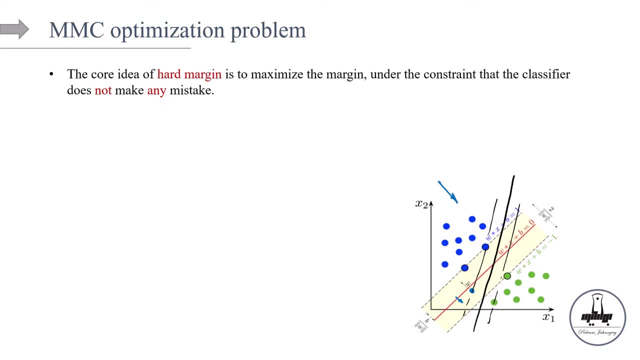 vectors, and this is going to be the new hyperplane, right? So with this new hyperplane, as you can see, there is no misclassification. So the core idea of the hard margin is that that hyperplane does not allow for any kind of misclassification. okay, 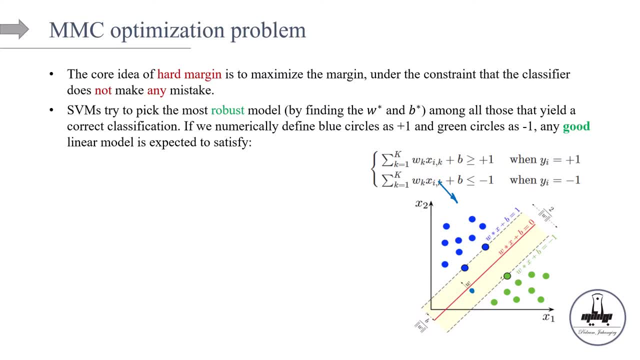 So SPM tries to pick the most robust model. specifically, the MMC try to pick the most robust model by finding the W stars and B stars. Guys, remember, at the end of the day, if I have the W stars and B stars, we are done. We can come up with a functional form for the F hat, which is a. 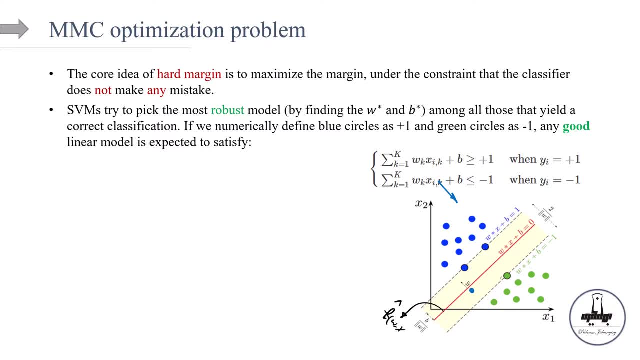 function of W and X. Of course W and B, there is a bias term in X right, And then we can make a classification based on this functional form, And so MMC tries to pick the most robust one among all those classifiers that yield the correct classification right. So now let's see. 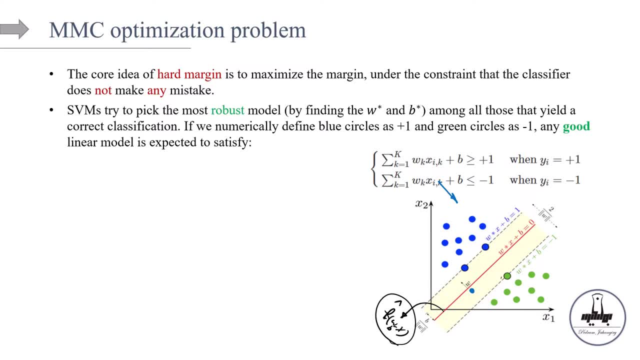 how it's done numerically. So if we numerically define blue circles on the margin as plus one and the green circles as minus one, so here the blue circles are plus one and the green circle is minus one- then any good linear model is expected to satisfy the 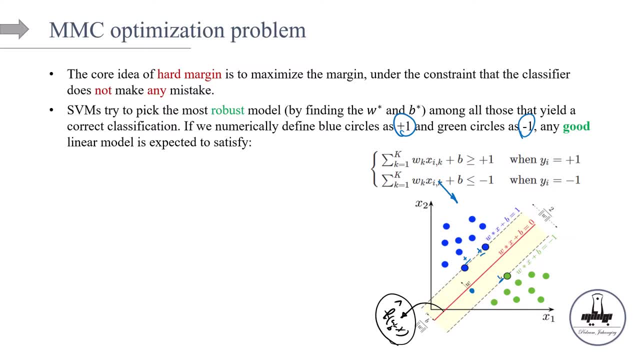 following constraint, right? So the idea that we use plus one or minus one, this is just for mathematical convenience. You could have used zero one, You could have used plus five minus one, But just for mathematical convenience we're going to use plus one, minus one and you will see the 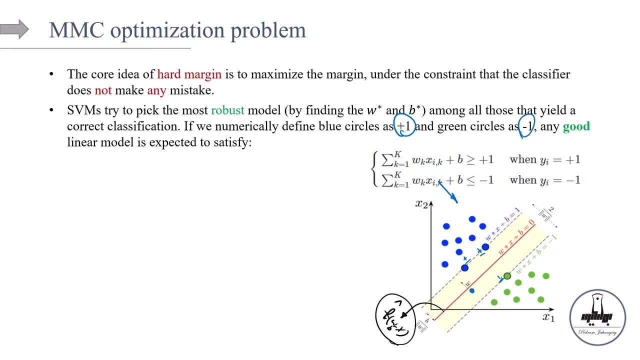 reason why we use this plus one, minus one. With that, let's do some calculations here over the graph. So imagine, imagine that the. so this is the equation, this let's call this blue margin. so this is our blue margin right, And the equation for the blue margin is: WX plus B is 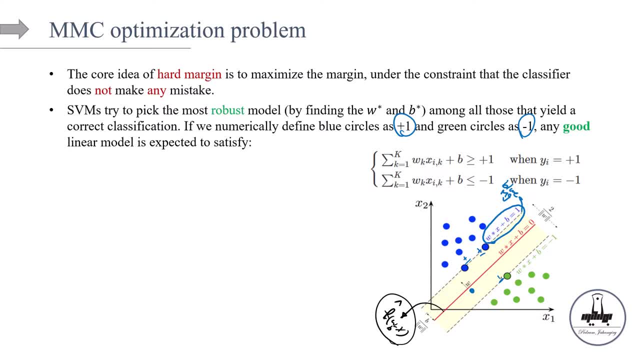 exactly equal to plus one. And the equation for green margin is: WX plus B is exactly equal to minus one right. And then if you want to calculate the perpendicular distance between the two, between these two lines, we know, we know the equation for that right. So if you watch the 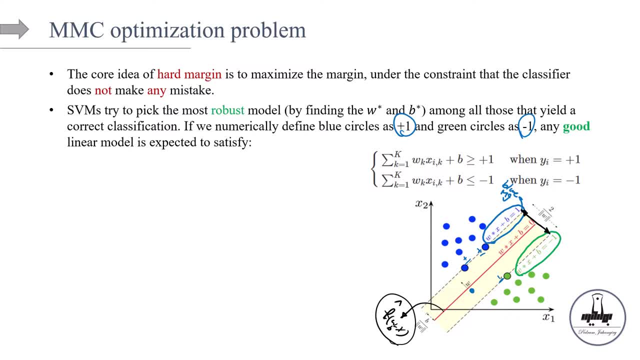 first part, part 23 of the equation. we know that the equation for that right. So if you watch this lecture series, you see that the perpendicular distance is going to be something like this: right, It's going to be the F hat of X, divided by the square root of W1, squared plus W2. 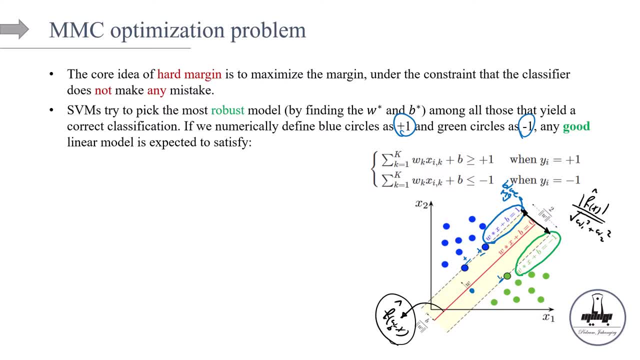 squared, okay, And then here, basically, the line in between is our hyperplane, and the equation for the hyperplane is: WX plus B is equal to zero. okay, So the numerator, the distance from the blue margin, of the blue margin, from the green margin, is going to be two, right, And then we need to divide it. 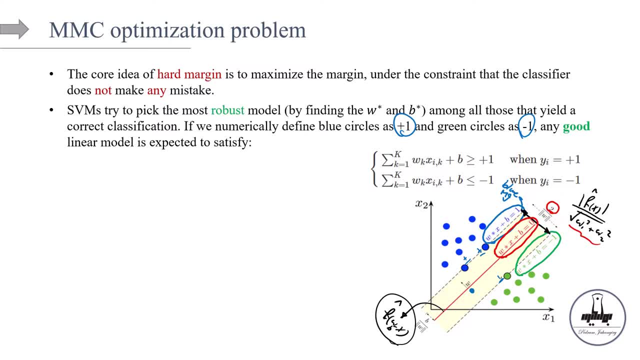 by some. this is our Euclidean distance right, The L2 norm of the weight matrix. So divided by basically the magnitude of weight, So the margin, the gap between the support vectors, are going to be equal to two divided by basically the magnitude of the weighting matrix right. 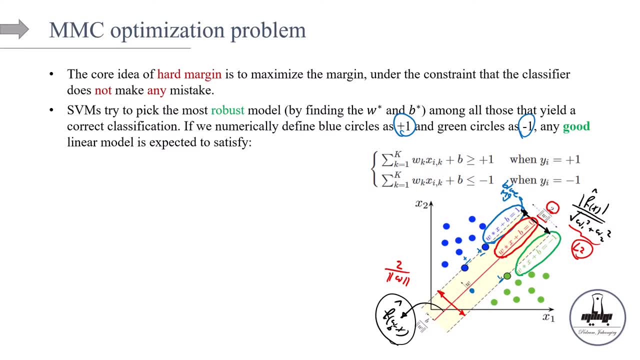 So in order to maximize this gap, this is equivalent to minimizing any function of W, right? So if I minimize any functional form of W, then of course that functional form needs to be strictly increasing and monotone and et cetera. But if I, in simplicity saying, if I minimize W, it's as if 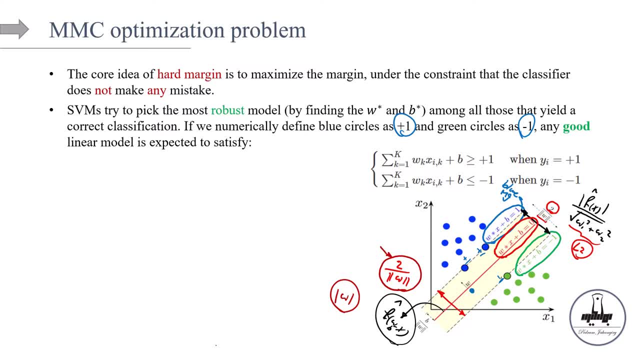 I'm maximizing two divided by W, right. So this is a way to minimize any function of W right. So this is number one thing that I want you to remember. Number two is basically look at all the observations, the blue circles, right? Remember the blue circles are labeled as plus one, So the idea is that all 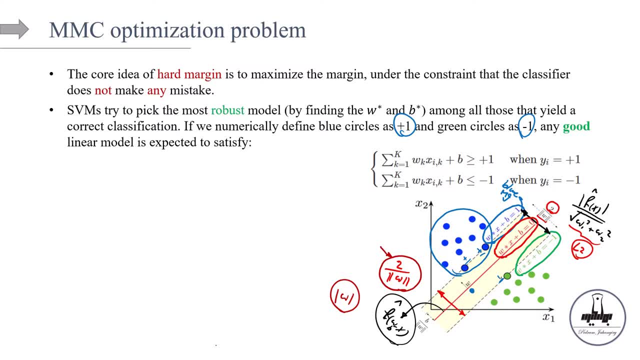 these blue circles to the left of the hyperplane are should have a distance larger than the one right. So how do we write it mathematically? We say, okay, if Y is equal to plus one, the blue circles, this should hold right. 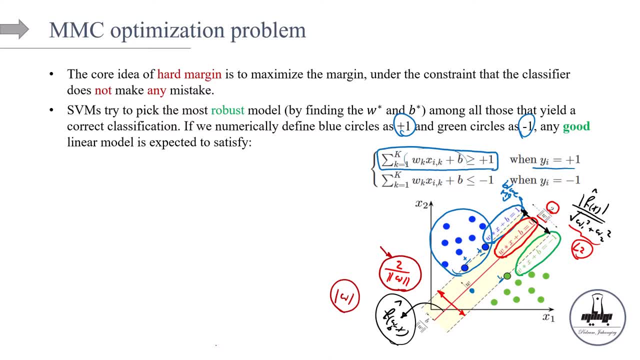 What is the first part? The first part is basically: if I plug these blue dots here, I get the distance. So it says that the distance from the hyperplane should be greater than plus one. So these are the blue circles, and for the green circles are all the observations to the right side of the hyperplane. 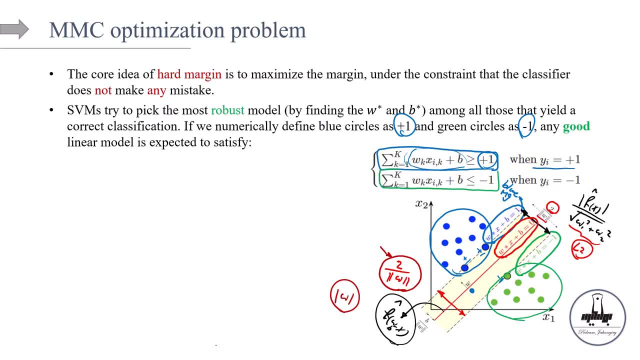 here, And the distance should be less than minus one, because we labeled these green circles as minus one right. So anything to the right should be less than minus one. anything to the left should be greater than minus one plus 1. okay then, now it's going to become more straightforward why we are. 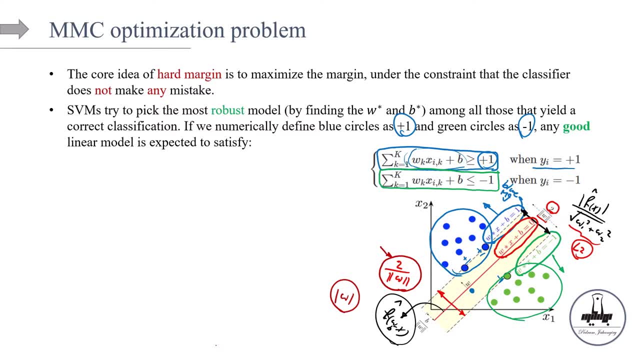 using plus 1 and minus 1. let's say I have two constraints, right, these are the two constraints. I'm gonna go ahead and write them using one single constraint, right? so just look at this one. if I go ahead, let me erase these extra things. if 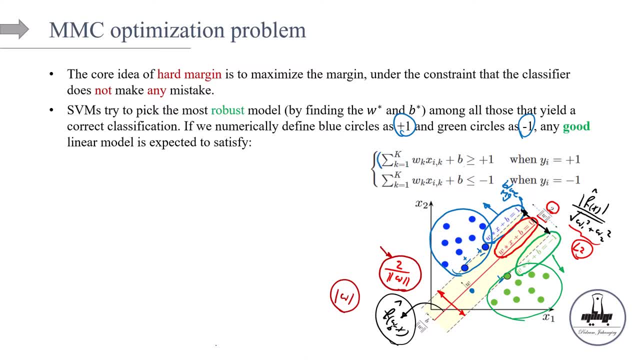 I go ahead and multiply the first constraint by Y. what I get- remember why I, for the first country, is constantly- is always positive, positive 1. so basically nothing is going to happen, right? if I multiply both sides by plus 1. so I have this one greater than plus 1, right? so the first constraint is going to remain. 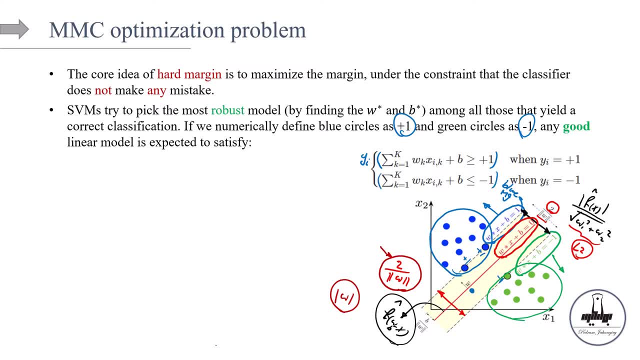 unchanged. what if I multiply the second constraint by Y? I remember why I, for the second constraint is going to be equal to minus 1. so I multiply both sides by minus 1. so if I multiply both side of this equation to minus 1, so I get this. 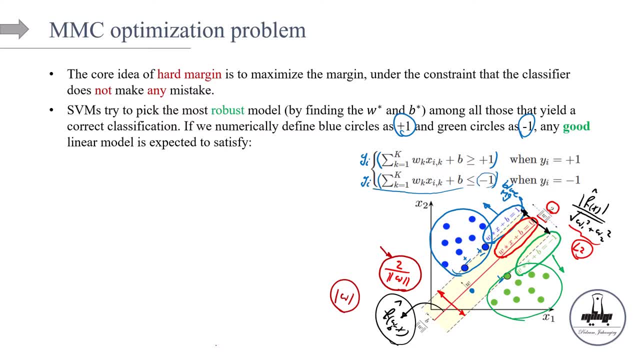 part, and this part, multiplied by minus 1, is going to be plus 1 and the direction of the inequality is going to change right and as, if you pay attention, both of these constraints are going to be narrowed down to one constraint, right? so overall, we have two things. we are maximizing the gap, which is equivalent. 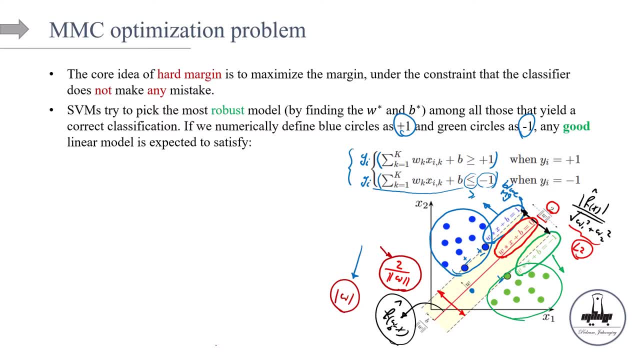 to minimizing the functional, the monotone function of weight and over this constraint, which we reduce them to one constraint. so let's, let's sum it up, sum it all and write the optimization problem. so here's the optimization problem: we are minimizing the 1 divided by 2 of the L tumor of. 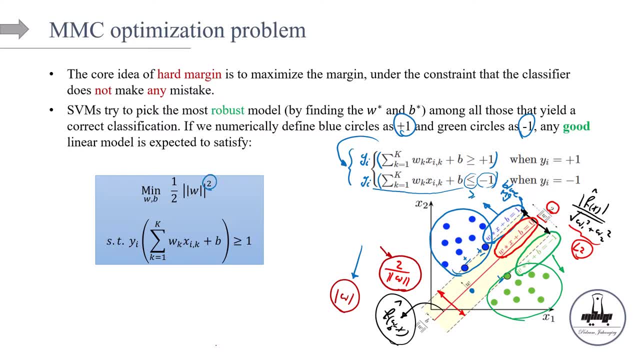 weights to the power of 2 right. so this is just a monotone function of W right. and again, for mathematical convenience, we do 1 divided by 2. multiply this W to power of 2, because down the road if we take gradients, so these 2 is going to cancel out with it. 2 in the denominator. 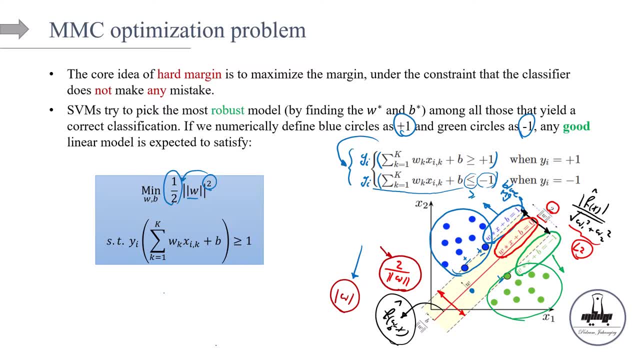 and it's going to give us easier time to calculate it, to look for a closed-form solution, right, and so we are maximizing the gap by this optimization problem. and what is the constraint? so why I multiply? this should be greater than 1 and, as you can, as we talked about it here, this constraint already has these two. 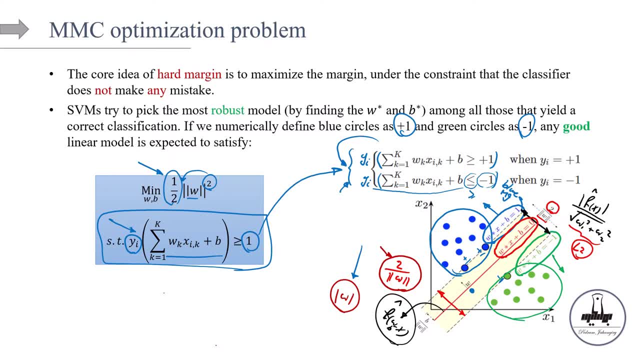 constraints inside it. so that's why we do the y, we define. the y is equal to plus one and minus one. so that's just for the mathematical convenience, okay. there's one thing that i want to emphasize in mmc: maximum margin classifier optimization problem. the idea is that we can either find we 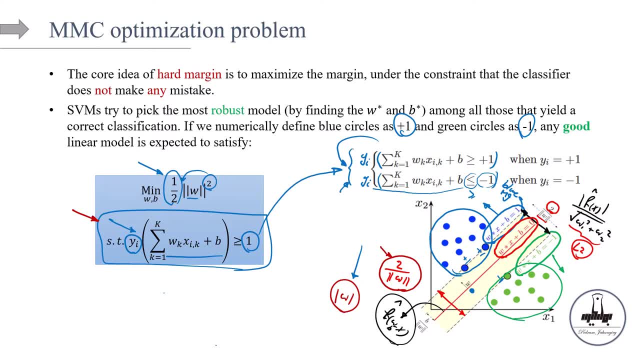 can either satisfy this constraint or not, and this constraint means that we are not allowing for any kind of misclassification. remember, all the observations should be to the right side of the hyperplane, to the correct side of the hyperplane, right. we are not allowing for any kind of 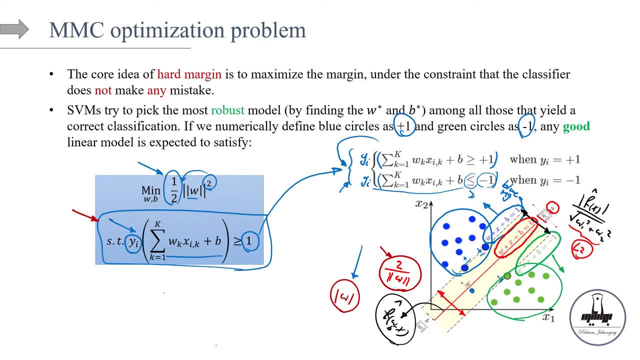 misclassification within the margin right. so there is either an answer for this optimization problem or no. if there's an answer, we can come up with a close-form solution. if there is no answer, we have to sacrifice the idea of using hard margin, and so we are going to expand this idea. 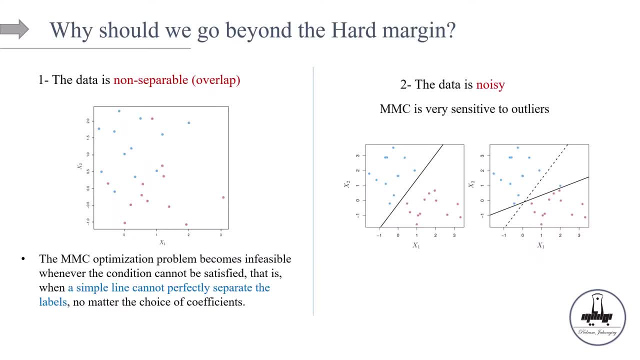 of hard margin, you the soft margin, okay. so why should we go beyond the hard margin and sometimes, why we have to go beyond the hard margin? there are a couple of common cases that we're going to explore here. number one reason is that maybe the data is non-separable. right, there's overlap between 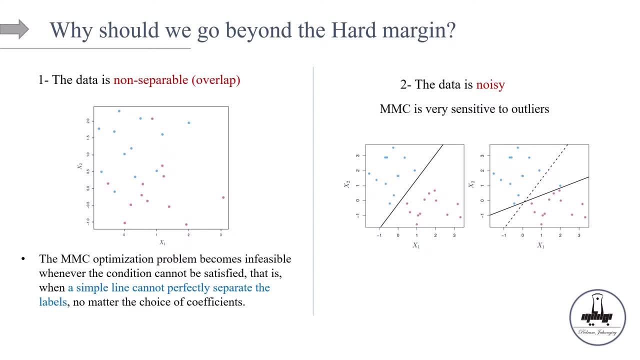 observations. so between classes. imagine, in this classification problem we have x1 and x2 and, by the way, in all the examples that we have in this set of slides, as you can see, the x1 and x2 are all the features that we have in this set of slides. so we can see that the x1 and x2 are all the features. 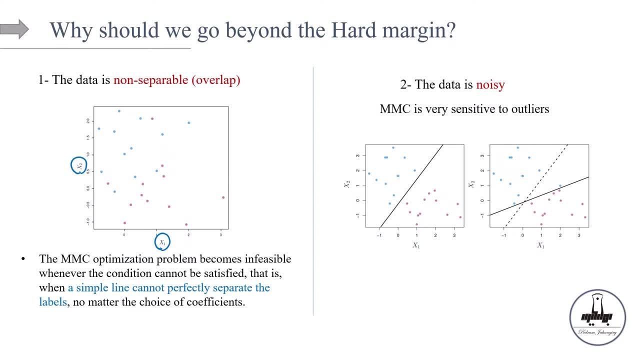 are scaled right and the reason that we are going to scale the features is because we are calculating a distance between observations, and the rule of thumb is that when you're calculating distance- either euclidean distance, manhattan distance- in any kind of machine learning model, we would be. 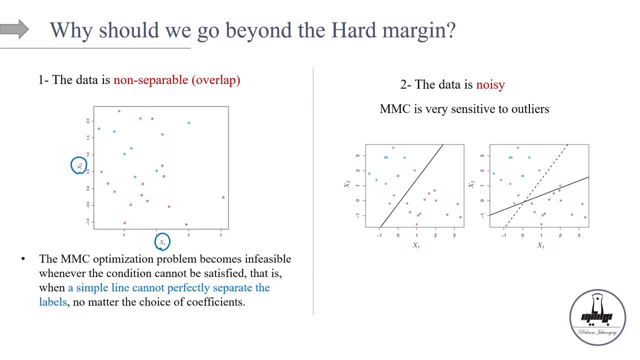 better off to scale the features, because we want to make sure that the the features. we're comparing apples to apples when you're calculating the weight. okay, so let's look at the case where the data is non-separable. so i want you to pay attention to the red uh, to the yeah to the blue circles versus. 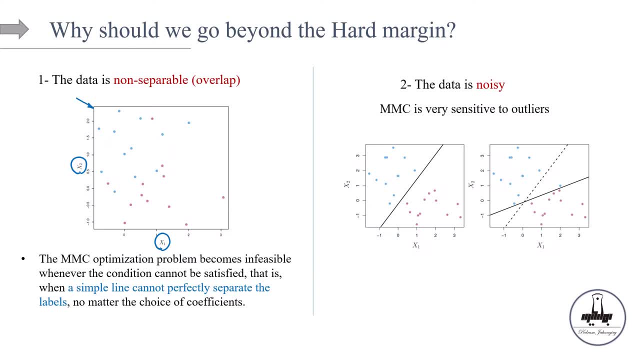 let's call them purple circles- and try to come up with the hard margin, try to come up with a maximum margin classifier. so can you find an answer? whatever you do, you cannot find a solution right. so simply the optimization problem that we saw on the previous slide, that's that, become invisible. 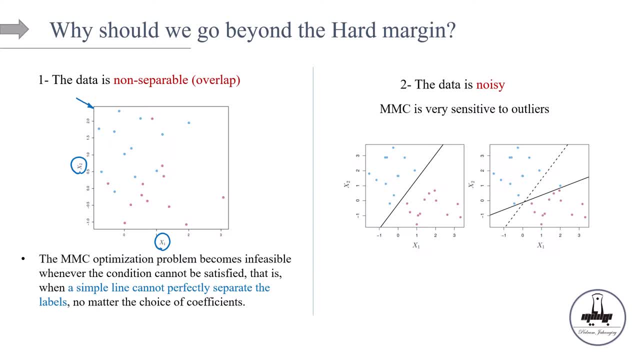 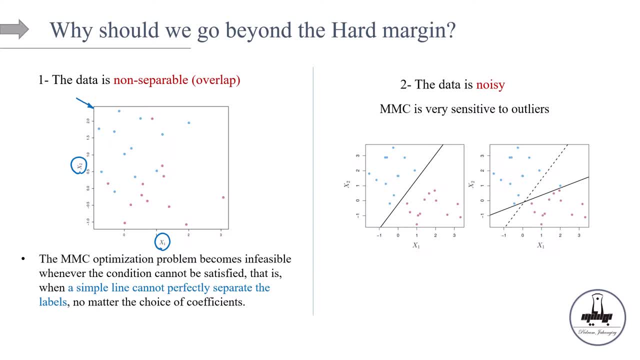 no matter how we rotate, how we change the coefficients, how we change the b, how we change the w's right. so if i do anything like this, there's going to be misclassifications here and there. right, so to simply: when the data set is non-separable, the, the hard margin is not. 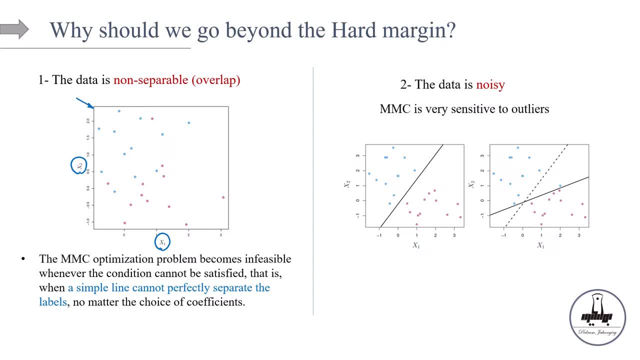 going to work. so we have to ex, we have to just use soft margin instead of hard margin. so this is one case. another example is when the data is noisy, even though we can't find the mmc, we can't find the maximum margin classifier, but we will be better off if we use the idea of 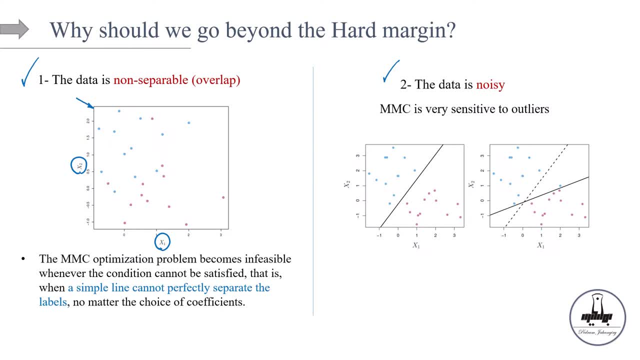 soft margin instead of hard margin. let's look at this example. imagine we have blue observations and russia's purple observation and, as you can guess, this is going to be our maximum margin- hard margin- and this is going to be our maximum margin- hard margin- and this is going to be our. 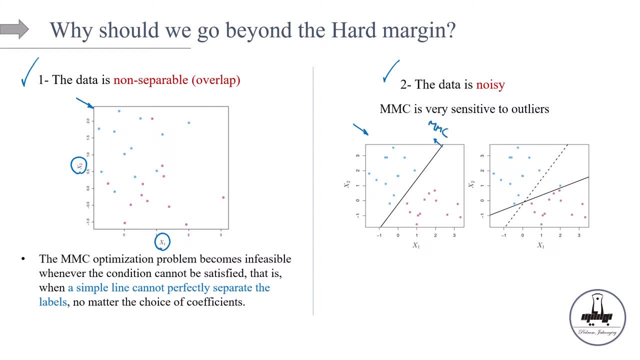 hyperplane right maximum margin classifier. so, and let's say these are the margins, so we have this margin right. so how many support vectors do i have in this example? one, two, three. so we have three support vectors and this is our maximum margin. so it seems that 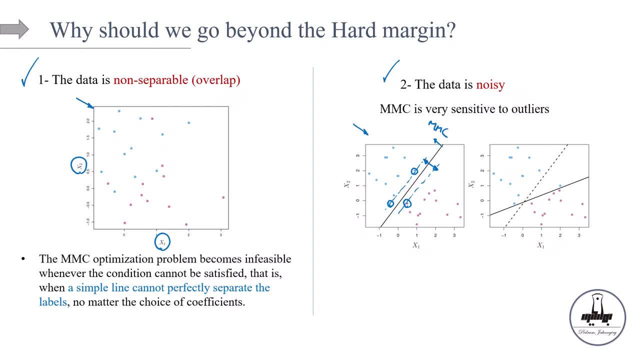 the previous optimization problem that we saw on the previous slide. it does have a solution, right, but the idea is that if you use a hard margin, the hard margin is going to be super sensitive. it's going to be very sensitive to outliers, right, uh, or to the to the observations. 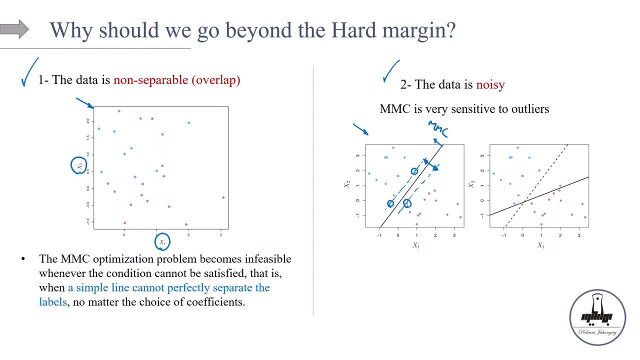 close to the hyperplane. so let's, let's, let's look at an example. imagine we have another blue observation just here. look at, let's look at the second graph. so if i add a blue observation here, then, in order to satisfy those constraints, my mmc is going to rotate completely from this line. 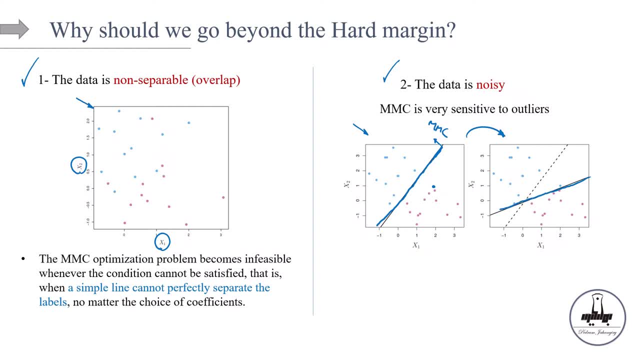 to this line. you see, so this is a huge rotation in terms of, you know, w1, w2 and etc. right guys, again, this mmc is going to be completely identified by finding w star 1, w star 2 and b star. so if i rotate these w stars i will get another mmc. and here, if, if you want to stick, 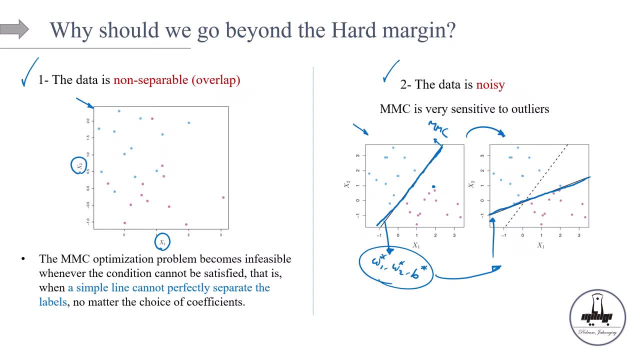 to that mmc hard margin, if you want to make sure that we are not allowing for any kind of misclassification. this mmc is going to shift dramatically. so, as you can see, it is sensitive to these points. right, so we don't necessarily like this one because because maybe one simple observation, one single observation, is going to rotate. 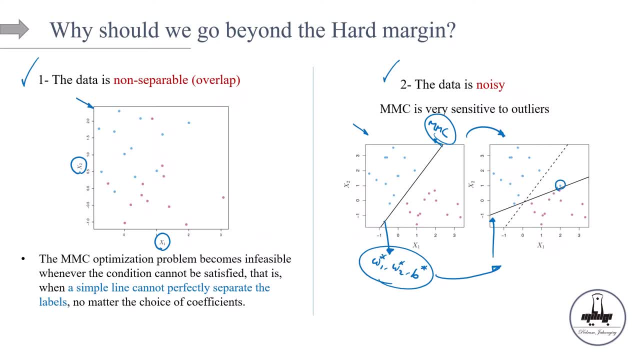 our mmc a ton. so in order to get a more robust model, maybe we need to sacrifice, somehow, get rid of this observation, you know, give some slack to the model, use soft margin instead of hard margin. so that's the idea of using soft margin versus hard margin. so let's talk about 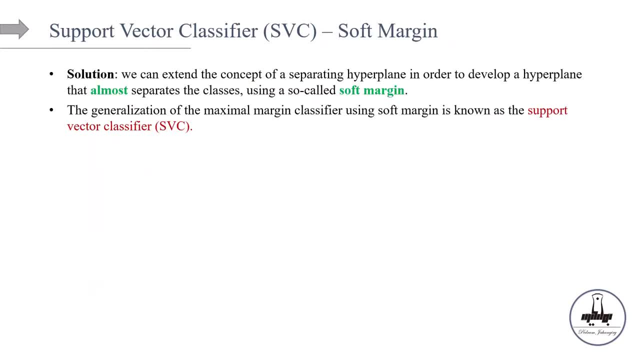 it in more details. so what's the solution to the problems that we discussed in the previous slide? the solution is: we can extend the concept of a separating hyperplane in order to develop a hyperplane that almost separate the classes using a so-called soft margin. so we have to go from 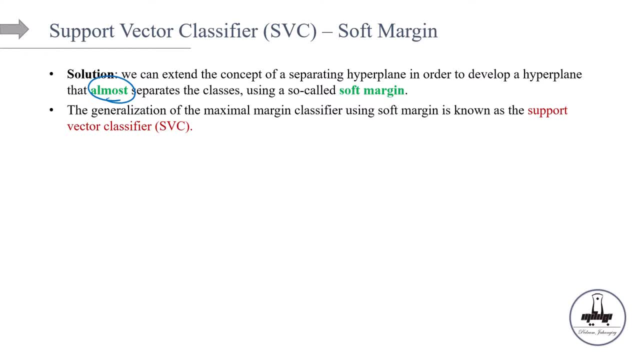 hard margin to soft margin in order to basically fix the issues that we talked about, right? so this generalization of the maximum margin classifier, the hard margin using a soft margin is also known as support vector classifier, svc. so remember, mmc maximum margin classifier is used for hard margin. 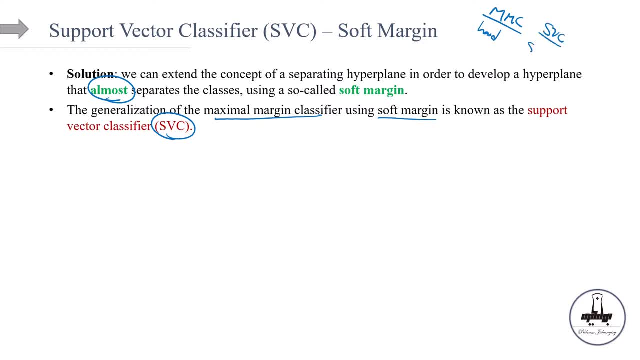 and svc is when we go from hard margin to soft margin. okay, so the core idea is that it could be front and back. after all, the different variables have fica e and vice versa. okay, so so normally, uh, a broad magnitude of the captivation factor, which is very high for the engineer. 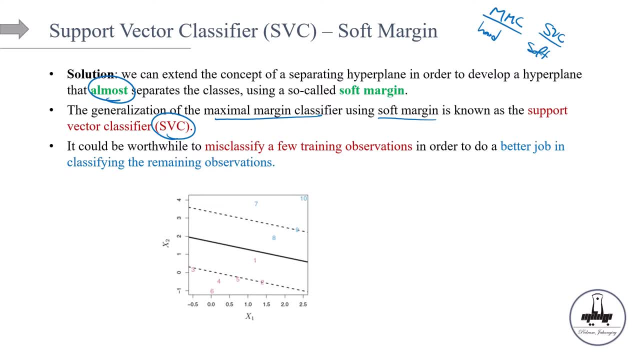 as a residual, we are now continuing the solution to the squared Teaching method. here is a Dashboard method. it's called the Dashboard method, our class blue right, So look at that. In this case I can't find the MMC right. So basically, 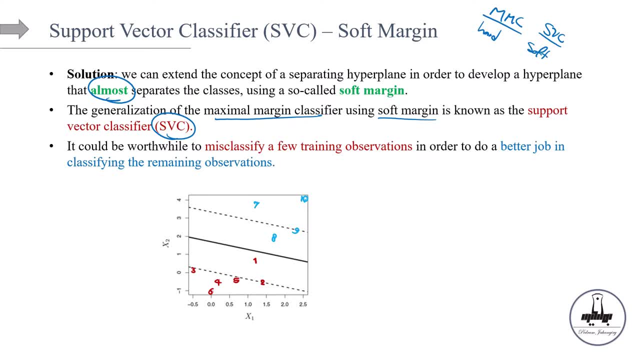 if I want to find the MMC, I should do something like this. So let's find the MMC such that it's going to maximize the distance from classes, basically the supporting vectors. So maybe we get something like this. Maybe this is a maximum margin. So this is going to be the hyperplane. 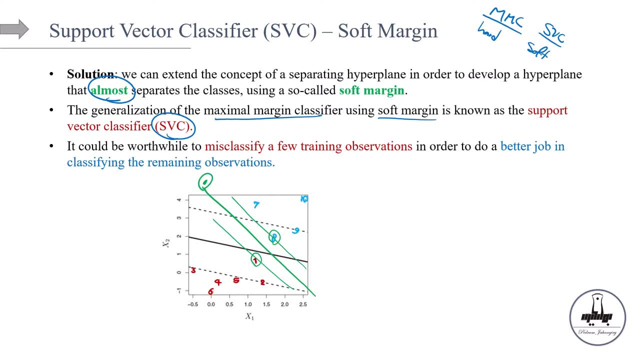 right, I label it as one right, But, as you can guess, this hyperplane is sensitive. It's sensitive to observations close to the margins, right, And we say that this hyperplane is less stable because it's using only two support vectors: this one and this one. Now, if I just 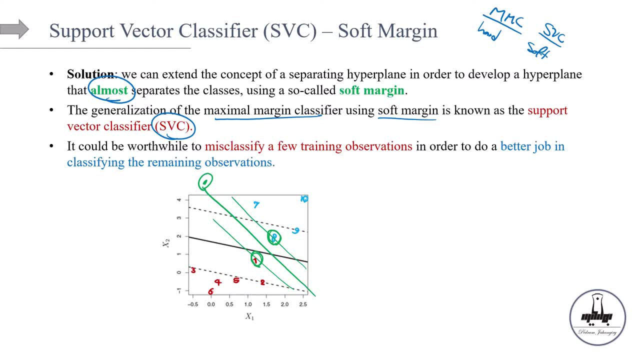 expand the idea of hard margin to soft margin, we can come up with something like this: This is going to be the classifier, This is our soft margin, And we are going to allow for a couple of observations to be on the wrong side of the margin, So let's label them, because here's the 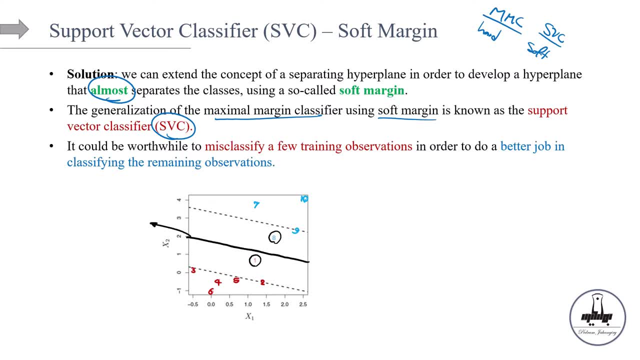 terminology is going to be a little tricky. So this is our hyperplane. hyperplane, This is margin. okay, And this is also margin. Now, if you pay attention, observations number 2,, 5,, 3,, 4, and 1 are on the correct side. 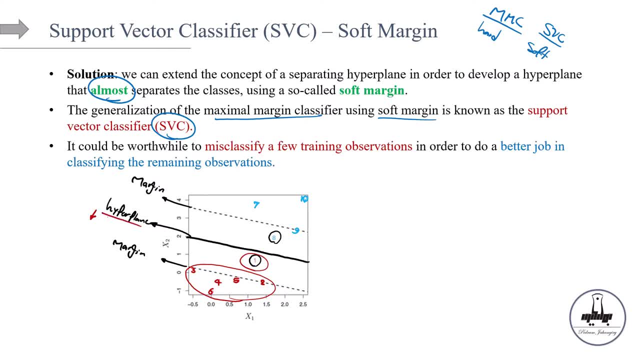 of the hyperplane right side of the hyperplane Observation 2,, 4,, 5,, 3, and 6 are on the right side of the margin as well. So correct side of the margin Is everybody following Okay. 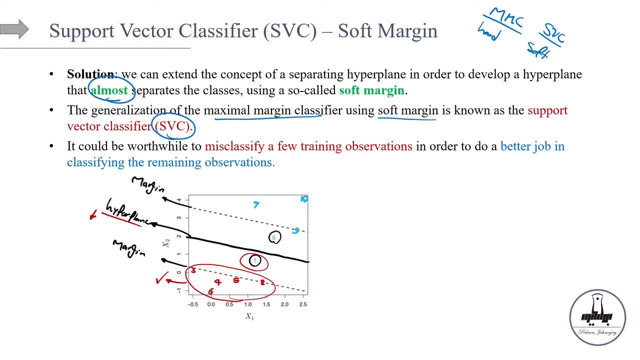 So these are on the correct side of the margin, but observation number 1 is on the wrong side of the margin. So wrong side of margin, but correct side or right side of hyperplane. So this terminology is going to become important. And for the blue observations, as you can guess, 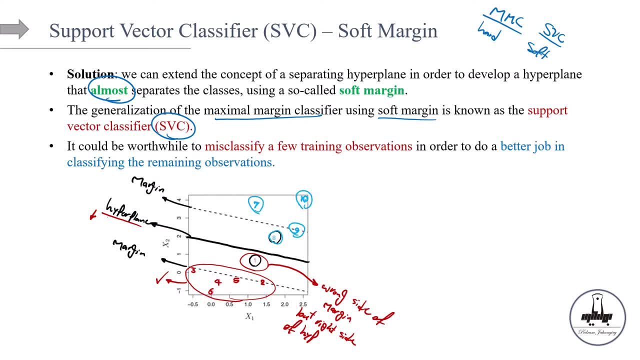 7,, 9,, 10, and 8 are on the correct side of the hyperplane, but observation number 8 is on the wrong side of the margin. So wrong side of the margin, okay, Because if this is a blue margin, 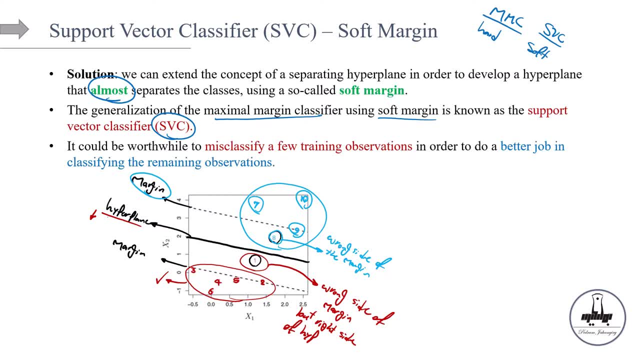 8 is on the wrong side of the margin. However, it's on the correct side of the hyperplane, right. So there is no misclassification in the traditional definition of misclassification going on here, because at the end of the day, we have a hyperplane. Let me highlight that hyperplane. We have a hyperplane, Anything above. 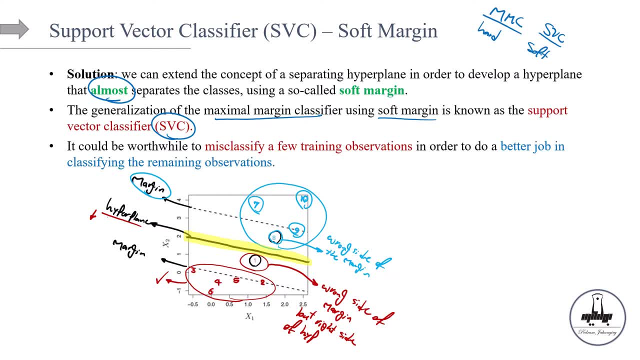 that we're going to call it blue. Anything below that we're going to call it red. So there's nothing wrong in terms of classification. However, there are a couple of observations, namely 1 and 8, here that are on the wrong side of the margin. okay, So if you remember in the MMC that restriction, 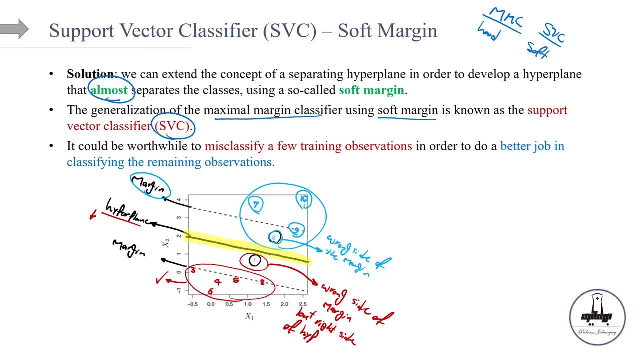 in the optimization problem does not allow for observation number 1 and 8 to happen right. So if you give the model some slack, if you tell the algorithm somehow just ignore number 1 and 8, it's okay for observations to be within the margin, to be on the wrong side of the margin. 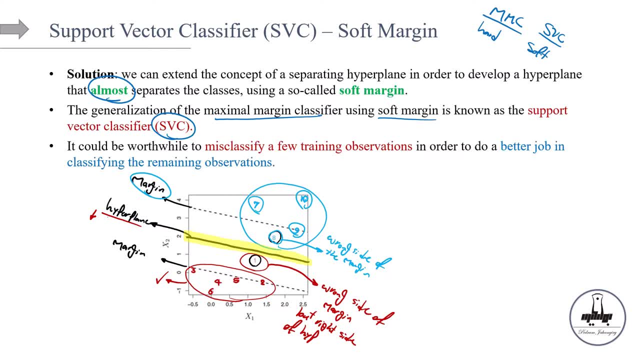 right. So if you say, if you somehow translate this idea to the computer, we're going to come up with this yellow hyperplane. And why do we use this yellow hyperplane? Because let's look at the support vectors. So this is going to be: if I'm using this, if I'm using this, if I'm using this. 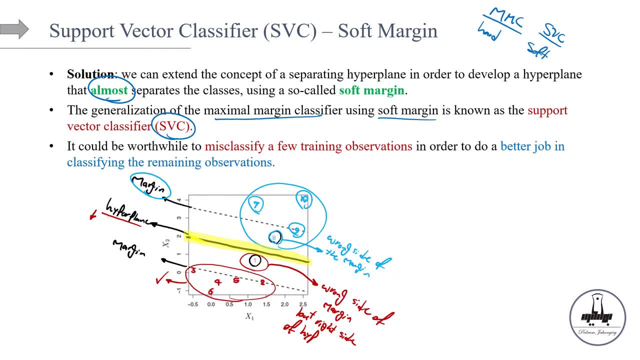 if I'm looking at the, this one, so let me use green if this is a hyperplane. So what are the support vectors? This observation, this observation maybe. 5 is on the margin. 3 is on the margin. 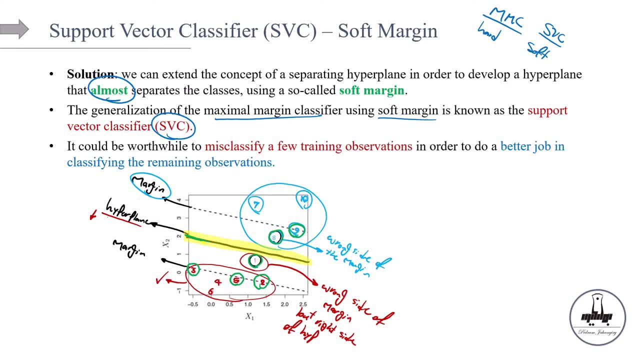 and all the observation within the margin. So we have observation number 1,, 2,, 3,, 5,, 8, and 9.. So 1,, 2,, 3,, 5,, 8, and 9.. These are our support vectors. 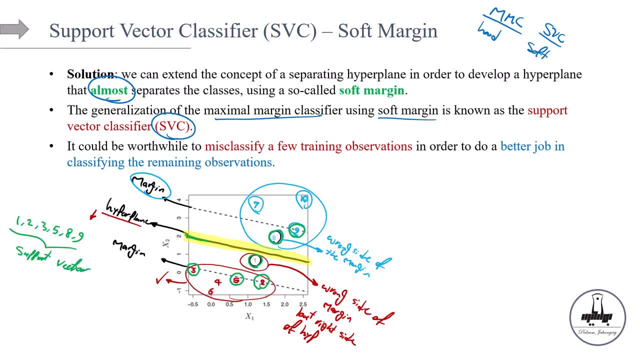 So now we have six support vectors compared to two support vectors if you use the hard margin. Remember, if you use a hard margin, we get something like this: okay, So let me erase them. So, having more support vectors, we're going to end up with more stable model. 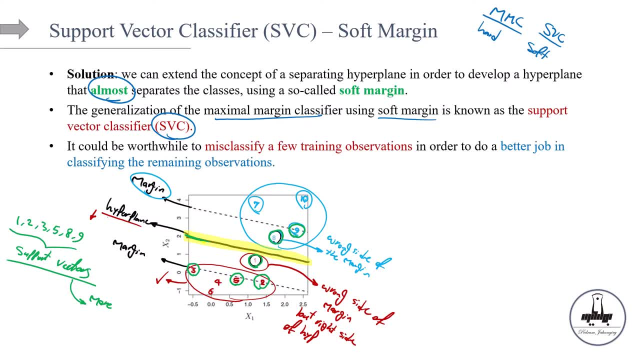 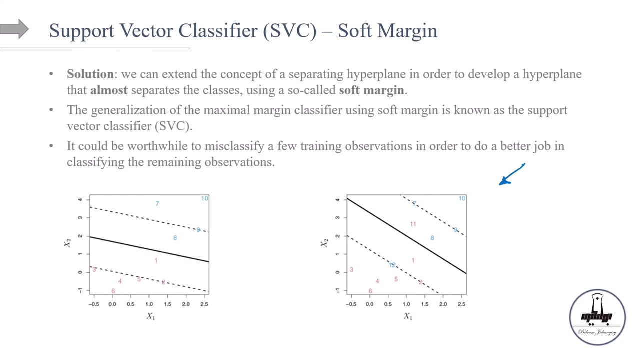 more stable, more robust in the train set, So it's going to perform better in the test set as well. okay, So this is one example. Another example that we cannot literally find the MMC solution is this one. So let's see, Is this one the one on the right right? So let's say I add two new. 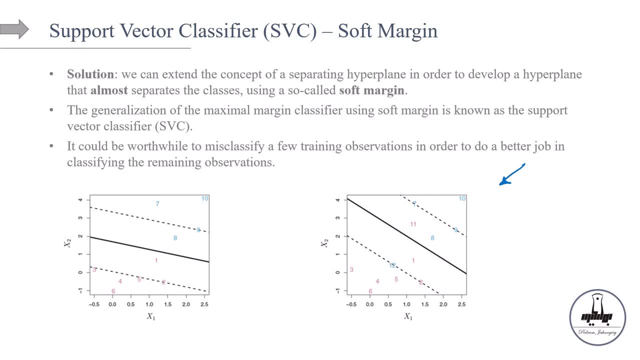 observations to the data that we explored in the previous slide. So let's say, I added this observation number 11 and observation number 12, okay, So let's quickly relabel the margin and hyperplane. So remember, this is going to be our. 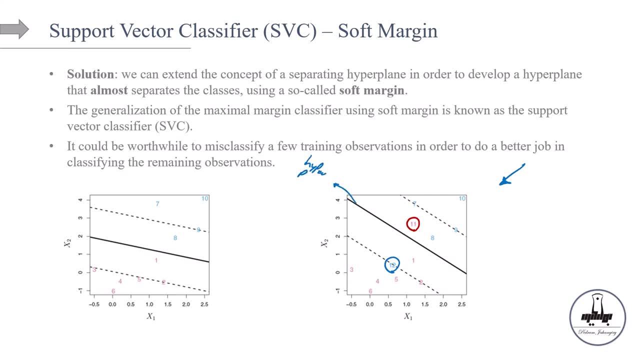 hyperplane. And these are the margins. Okay so, margin. Okay, so let's do some exercise together. So we have observation number 1. So let's use the right one, Right color. So basically, let's use red. Number 1 is on the wrong side. 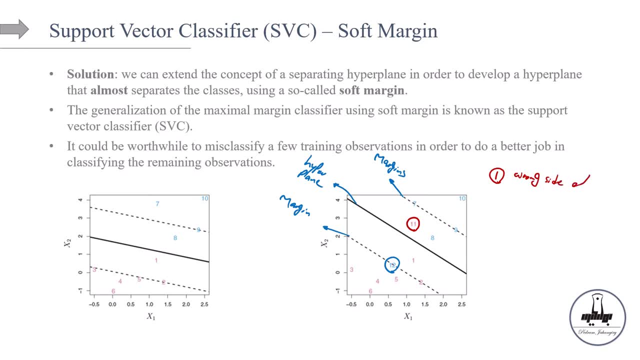 of margin right, Because this is a red margin. it's on the wrong side of the margin. However, it's on the correct side of the hyperplane. Observation number 8, the same story. Number 8 is on the wrong side of the margin. 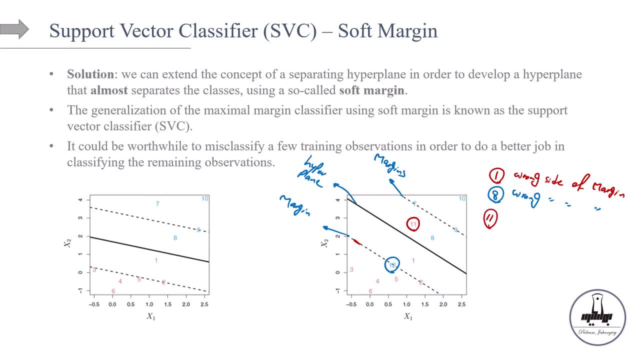 Observation number 9, is on the wrong side of margin. Observation number 10, is on the wrong side of margin. Observation number 11,, however, is on the wrong side of the hyperplane, So this is misclassified. Observation number 12, is going to be on the wrong side of hyperplane, right. 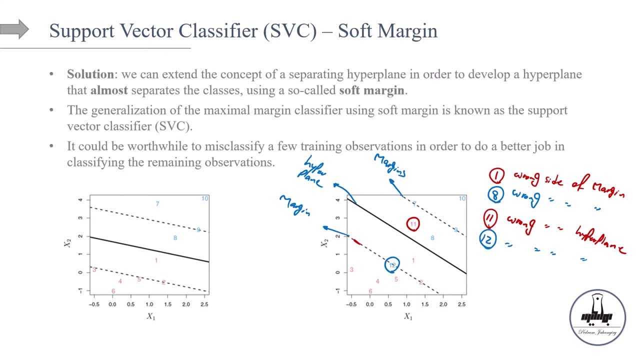 So 11 and 12, these are, let me highlight them. so 11 and 12, these are misclassified, because if this is a classifier, a classifier, if this is our support vector, classifier number 11 is going to be classified. 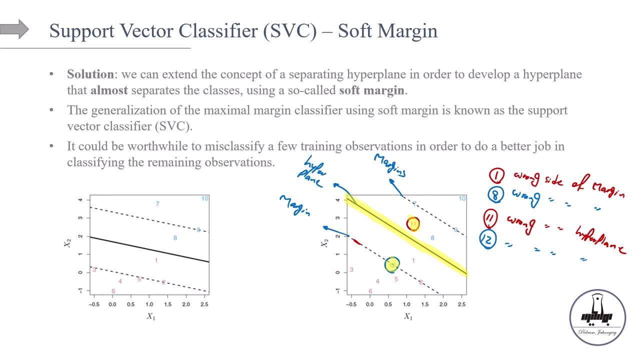 as blue, which is wrong. Number 12 is going to be labeled as red, which is also wrong. So these are misclassified. So the idea here is that we're going to allow for these misclassifications as well. right? So if you allow for these misclassifications, then you're using soft. 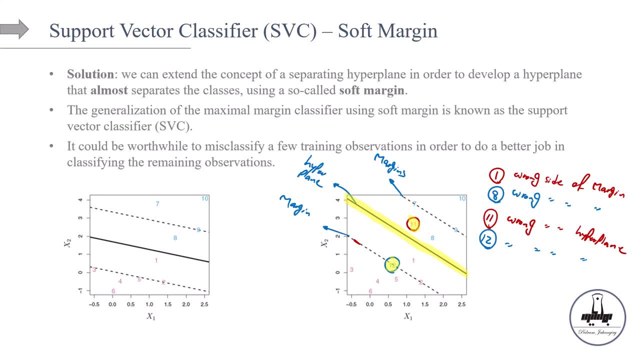 margin right. And so what are the support vectors here? At the end of the day, if this is our margin, we have one. well, let me use the right brush. So this is support vector. These are all support vectors, Okay, So in this case, I think, in this case, if you add this observation, 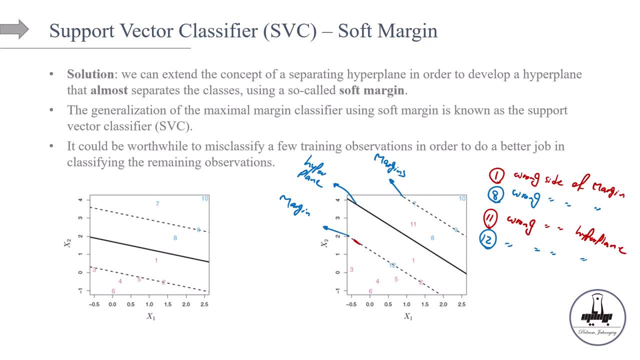 number 11 and 12, coming up with a hard margin is going to be almost impossible, Well, actually, it's going to be infeasible, right? So we cannot find a hard margin if we add number observation 11 and 12 to the data set, So we have to use the soft margin. Okay, Now let's. 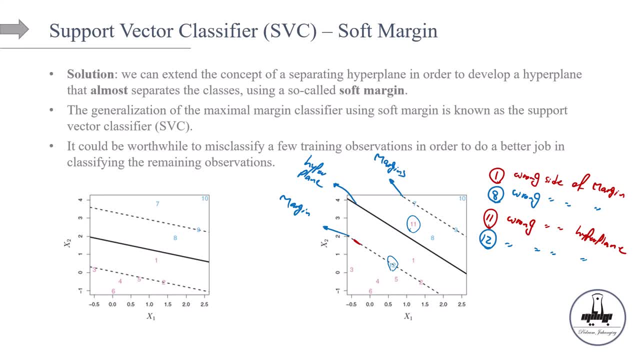 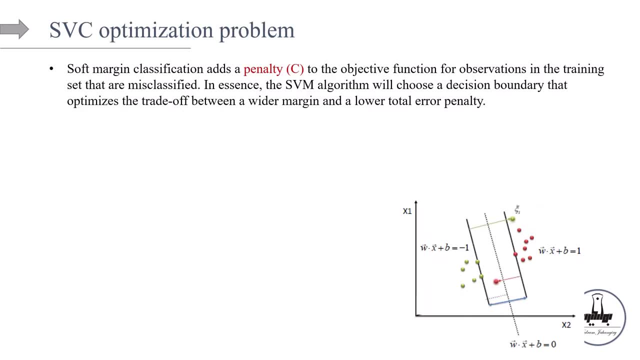 see how does the computer actually find the soft margin? What is the optimization problem for the SVC? So here is the SVC optimization problem. So the soft margin classification adds a penalty. So let's show this penalty term. Let's see To the objective function for observations in the training set that are: 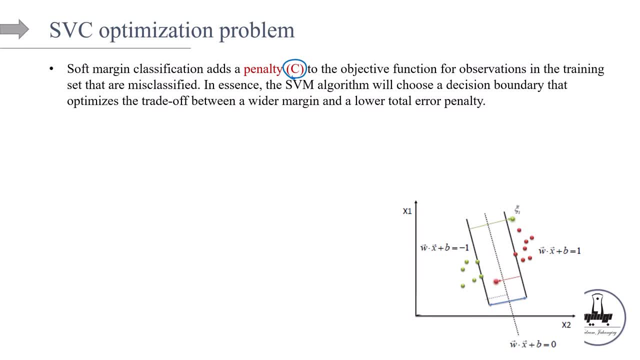 misclassified. So, in essence, the SVM algorithm- well, let's call it SVC- will choose a decision boundary that optimize the trade-off between a wider margin and a lower total error penalty. So the idea is that let's make that hard margin soft, in a sense that we allow for some. 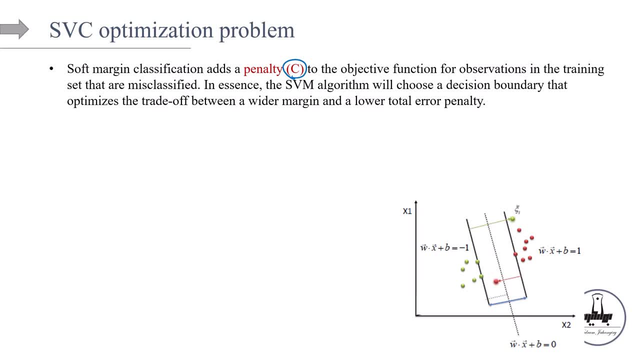 misclassification. But overall the error term of the model is going to decrease, right? So let's look at the constraint. So the constraints are going to be pretty much the same as the MMC, but we're adding the slack variable, So slack variable is xi, So let's call this xi. 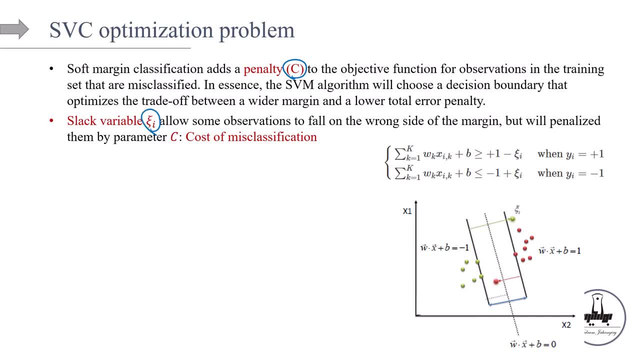 This allows for some observations to fall on the wrong side of the margin. okay, Not necessarily the hyperplane on the wrong side of the margin, But we'll penalize them by multiplying them to the penalty term whatever. So we define it as the c. 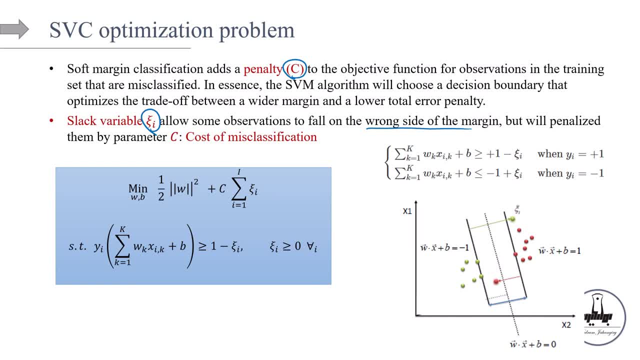 cost of the margin. So we'll penalize them by multiplying them to the penalty term whatever. So we define it as the c cost of the margin. So we explain it as the c cost of the margin. Here's the optimization problem. and as you pay attention, 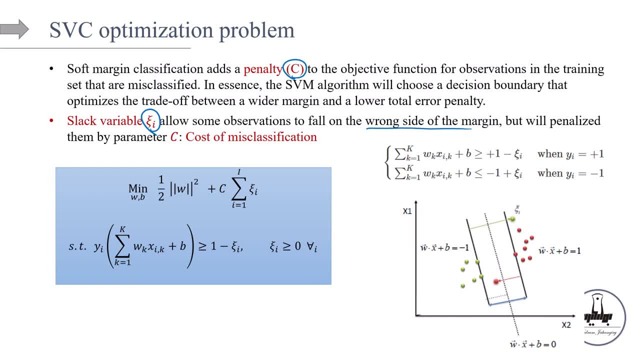 This optimization problem is very much similar compared to MMC, but the difference part is here. Let me use the highlight. this is: maybe this is a difference right, This part and this part. So let's try to understand what the algorithm is doing there. 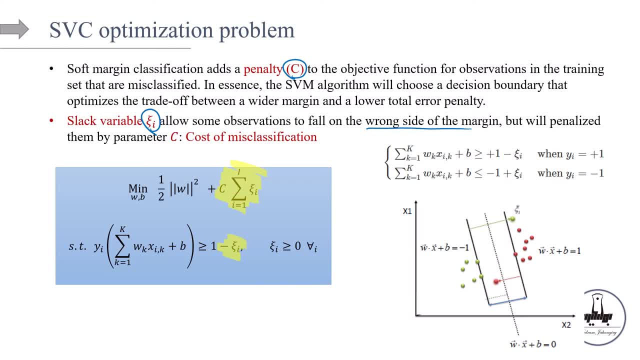 So these are the slack variables. These are the slack variables. This is a pretty normal message, So let's try to understand. let's actually look at an alarm function here. a bunch of those misclassifications. so paying attention to this example here. 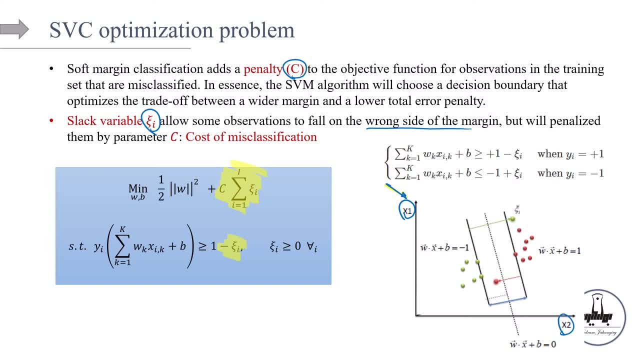 we have X 1 and X 2. there are two classes, class green, class red, and this is our hyperplane. this is margin and this is also margin right. as you can see, this observation is on the wrong side of the hyperplane. okay, so this means that 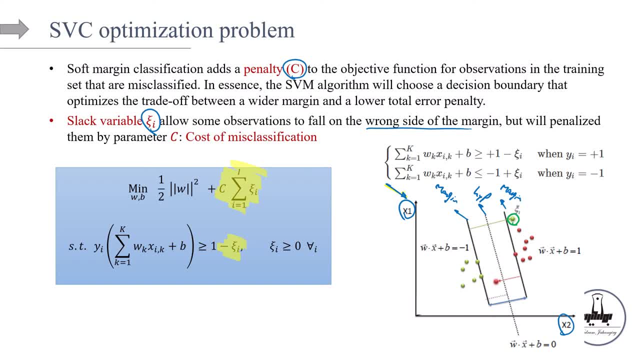 it's on the wrong side of the green margin as well, and this observation is on the wrong side of the hyperplane as well, so it means that it's misclassified, but it's not necessarily only these two points. so let's say I have red observation here, so the red observations is on the wrong side of the red margin. 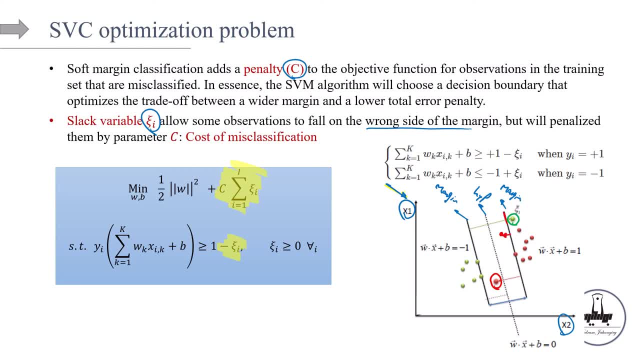 and then we can define this. so I for red, and let's say we have a green observation here. this green observation is on the wrong side of the green margin. so this is our zy for green here. so, as you can guess, these two new observations that I just draw, they're. 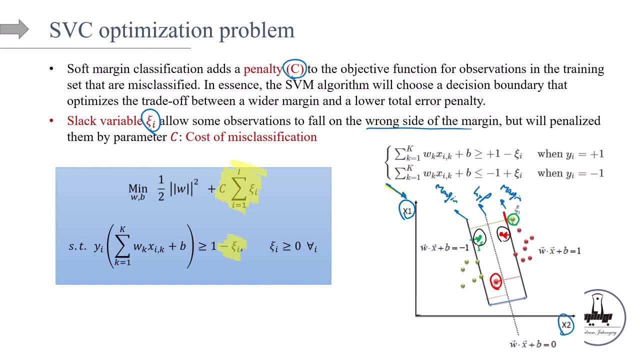 not on the wrong side of the hyperplane, but they are on the wrong side of the margin, so we need to give them some slack as well. we are going to allow for them. so it's okay to have these observations within the margin or dismiss classifications, but you're gonna penalize them, right, so we're gonna. 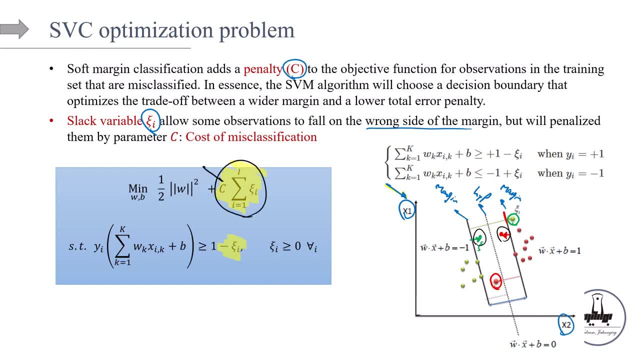 penalize those zys by multiplying them by positive, let's say cost function. right, it costs the positive seat number C. and so this is how we are going to penalize this minimization problem, right, because, remember, we were trying to minimize the objective function, but now we're adding some positive number to that, right? so this is going to 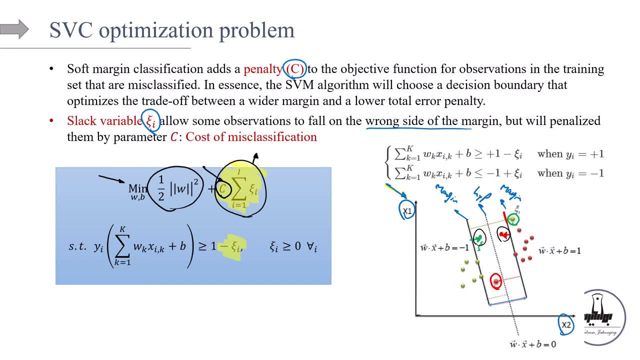 matter. what is? what is the actually? this C is going to become a one of the hyper parameters that we need to tune for for the SVC model. so this is the objective function. but what are the changes in the constraint? so the constraint, this part is pretty much the same, right. so the new part is this. so now we're going to say: 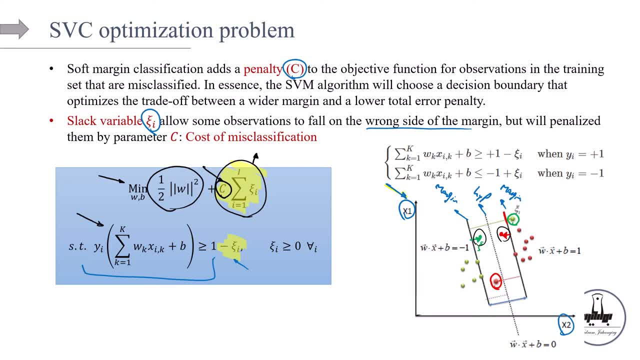 that, okay, you don't need to be exactly on the right side of the margin. I'm going to give you some slack, right, and that's how we're going to do it, right. so we say, okay, you don't need to be so. hey, you, this one, you don't need to be on the 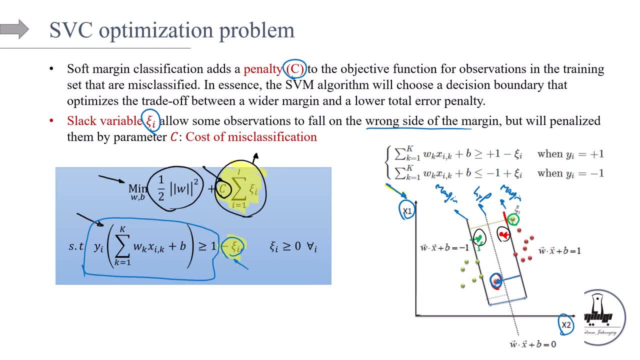 rights of the margin. I'm going to allow you to be within this margin, so I'm going to give you some slack, okay, so that's why we have one minus I on the right hand side. so this is the optimization problem for SVC, basically the idea of soft margin. okay, so let's wrap up this relatively long video by 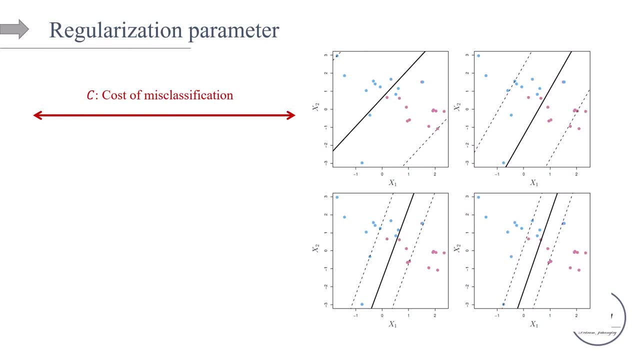 going over the regularization parameter in SVC. okay, so let me remind you of the optimization problem. we said that we are trying to minimize in SVC. you're trying to minimize this objective function plus adding some cost to the summation of these slacks, right, total slacks. so 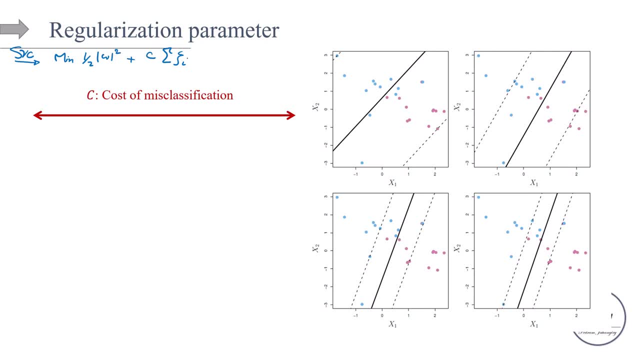 basically, the sum of slack means total distance of points on the wrong side of the margin right now. so we're going to use this C, we define it as cost of this classification and we treat it as a regularization parameter. this is going to help us control the bias variance trade-off, right? so let's see so imagine. 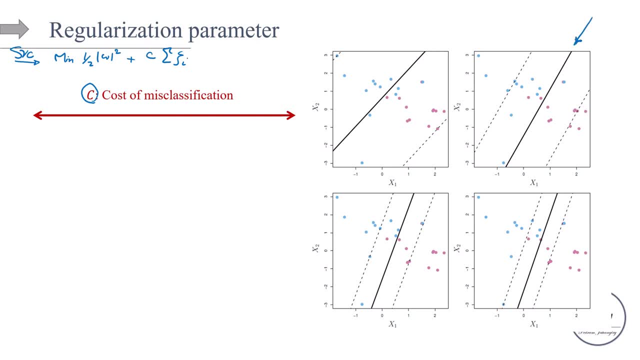 we have a data set right and we can have a very wide margin to a very narrow margin. okay, now let's see how does C affect the width of the margin? okay, so if C is a small? if C is a small, what does it mean? it means that we can. so 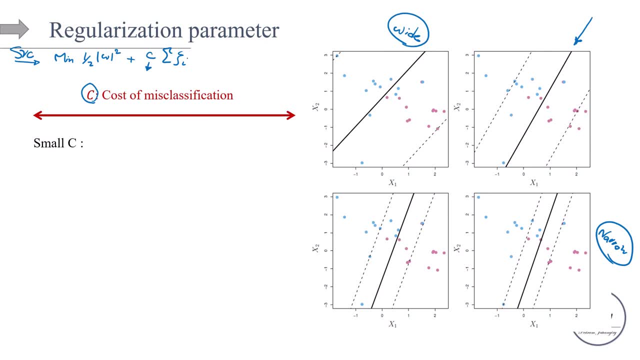 this C is a small means that we can have large slack- right, we can have lots of slack, right. if we can have large slack, it means that we can come up with a wider margin- right, so we can come with wider margin. so maybe we're here. C is a small. if C is a small, the margin is wider. so if you pay, 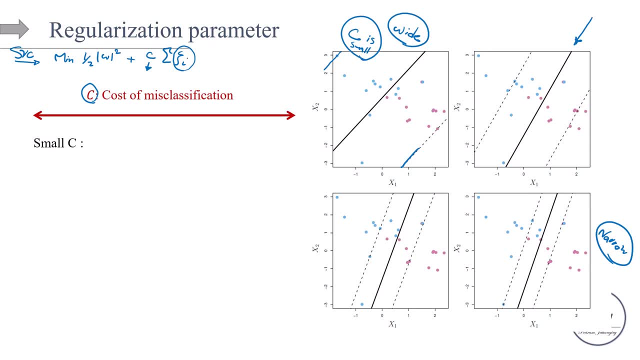 attention. this is, these are the margins and, as you can see, the margin is very wide. so if the margin is wide, the bias is going to be high. this is model bias, right? so because on average, maybe we are not finding the best classifier if we're not capturing a pattern in model, so the bias is going to be high. however, the 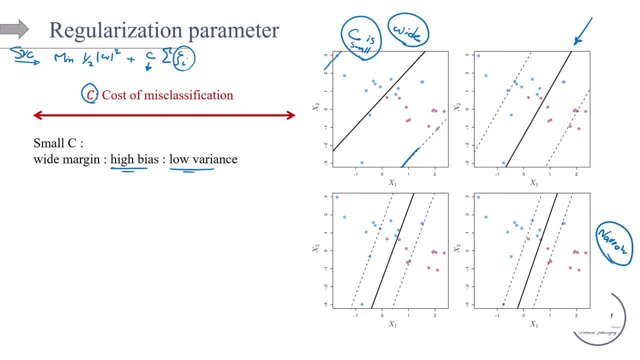 variance is going to be low. the model variance is going to be low, right, because if I use another sub sample there, well, using this very wide margin, the hyperplane is not going to change that much, right? so the it's not going to rotate that much now. if the C is large, so let me use red. so if C is large, then 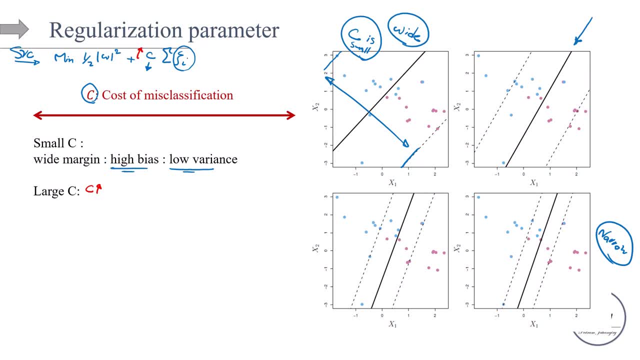 because this is a minimization problem. the algorithm is going to try to reduce these slags, right? if you want to reduce those slags, we have to come up with narrower margins, right? so let's say, maybe we are here, so here C is large. okay then, because we're not allowing for the sum of the total. the 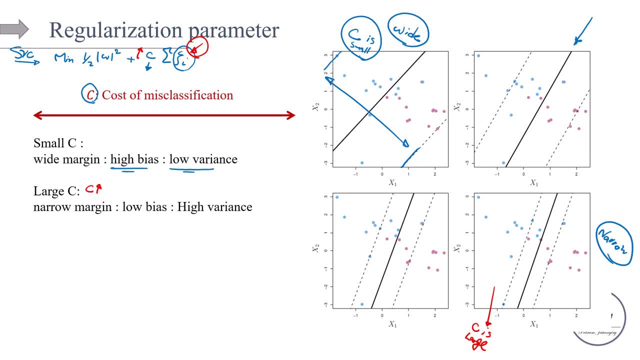 distance of the points on the wrong side of the hyper plane, on the wrong side of the margin. so basically, these slags, the summation of this slag should not be that high. so for that reason we need to have a lower margin, lower gap, right, let's say narrower margin. so if you have 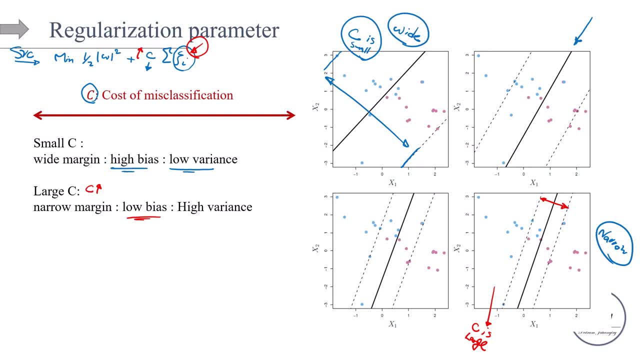 narrower margin. the model bias is going to be small because on average, you're hitting at the target where you're capturing the pattern. but the model variance is going to be large. right, because if I use another subset, you know if I use another. basically draw from the, from the, from the population or from the. 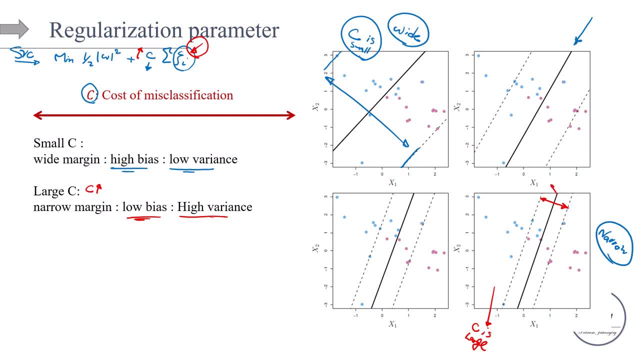 train set. this line may rotate a lot, okay, so maybe it goes through this one, this one and it's, etc. okay, okay, so inert. so if you, if you need a refresher in terms of what is model bias, models, what is model variance, please make sure that you watch the. 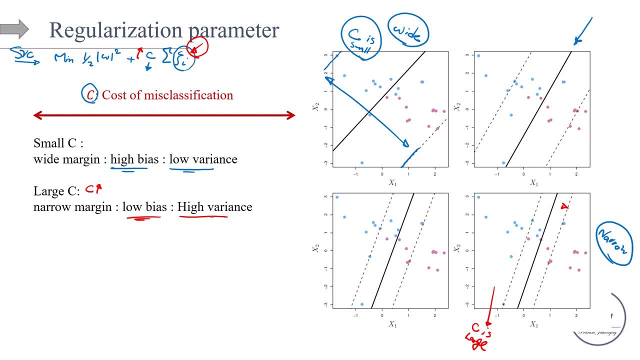 previous videos on this and this play YouTube playlist. okay, basically, you can follow. you can watch part 4 of this video if you want to watch part 4 of this video. 5 of this machine learning concepts lecture series, where I talked about the details of what is model bias, what is model variance. okay, all right, so that 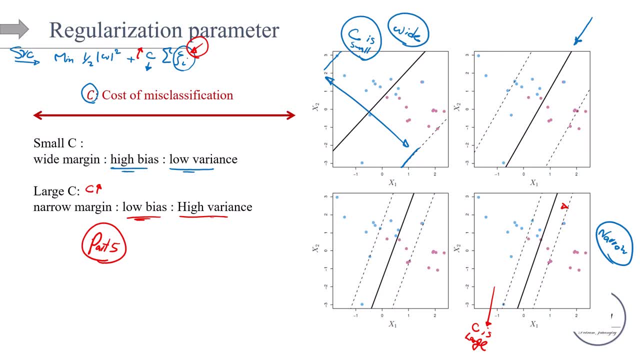 was it this? so so far we talked about the motivation of SVM and we saw the how. what is the algorithm behind SVM? in classification? we started with hard margin- we call it MMC- max margin classifier- and we said that sometimes there is no solution to the problem of SVM. and we said that sometimes there is no solution to the problem of SVM and we said that sometimes there is no solution. 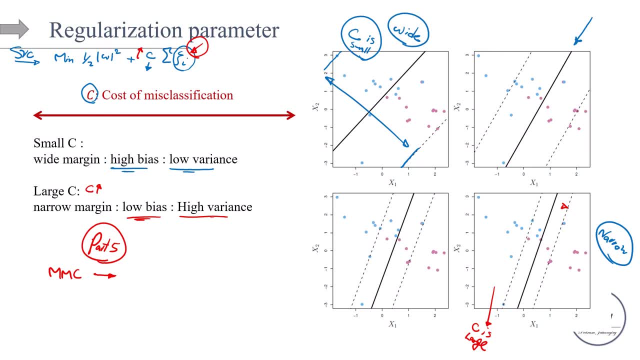 to this MMC problem and sometimes we want to get a more robust model. we have to go from the idea of hard margin to soft margin, so we call it SVC, and in the next episode we're gonna see that even sometimes we cannot use a soft margin concept alone and we have to even extend the idea of soft margin to some other.